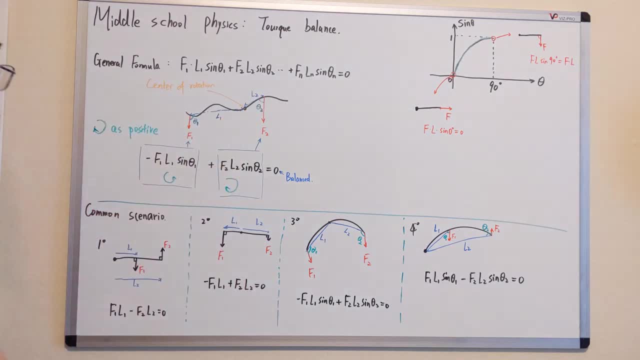 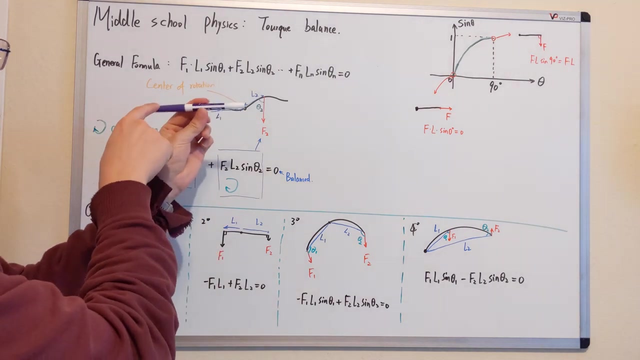 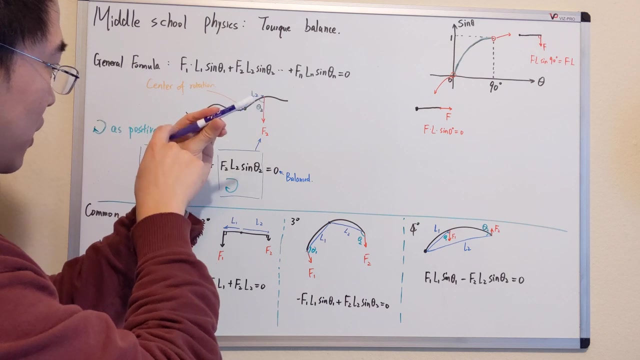 Here's a line. The length of the line will be L1.. And the angle between this L1, line of L1, and the direction of F1 will be theta 1.. And if you try to imagine that intuitively there's a center of the rotation, you tilt it this way, then you can think you will find out that this pen or this lever will rotate. 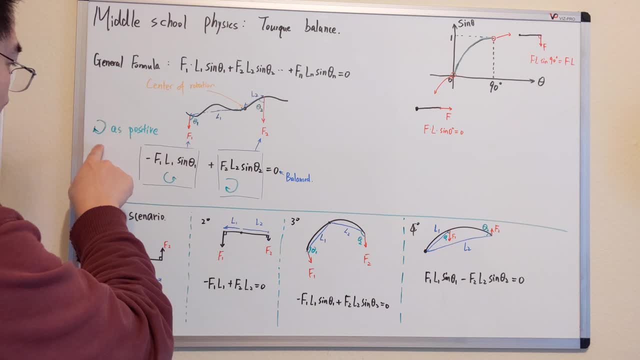 Now for the counterclockwise. since we defined the positive direction as clockwise, then this term should be negative. So this way we have negative f1, l1, sine, theta, 1.. Similar idea: we apply F2 here and connect the center of rotation with the point where the force is active. 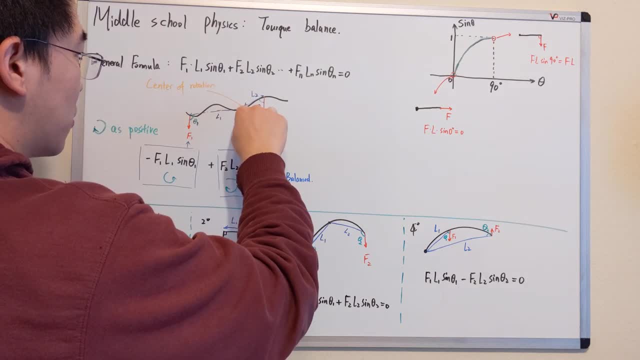 Here is L2, and the angle between L2 and the force F2 is theta 2.. Then we apply a conclusion. First we want to get the x of Love voucher loop-straight, which is calculating the lowest angle of l2 plus the хочетve for f2.. 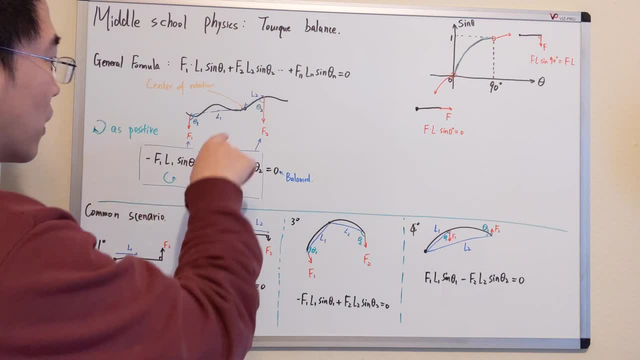 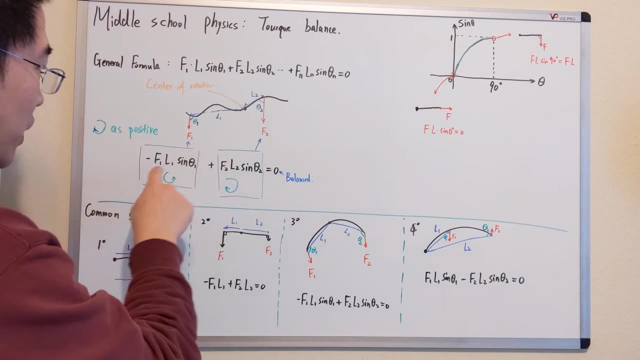 That'sale to 2.. Then we apply a culminary% and we plug f1.. Then we defined again, as we said, this one: if we apply force here, it will go clockwise, which is positive. Then we ended up having this torque balance equation. 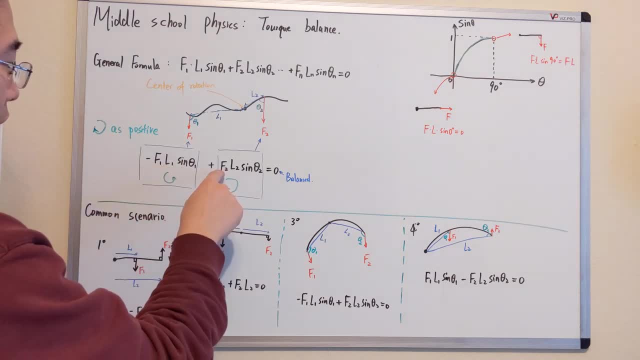 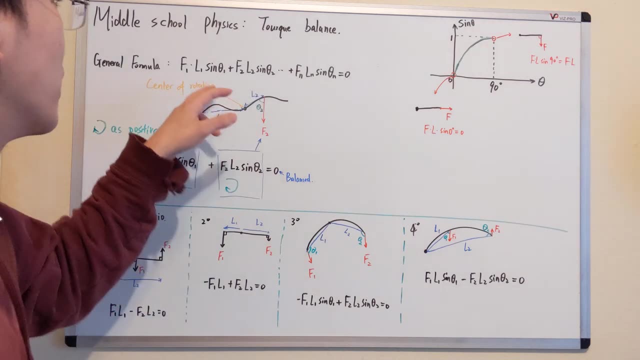 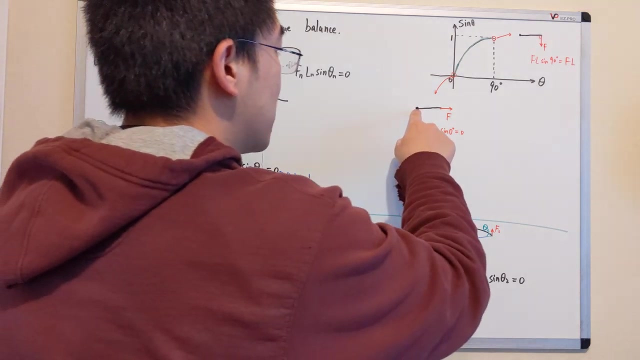 negative: F1L1 sine theta 1 plus F2L2 sine theta 2.. So intuitively, let's think about what the sine theta contribute to this equation. So let's imagine a scenario: We have a center rotation on one end. 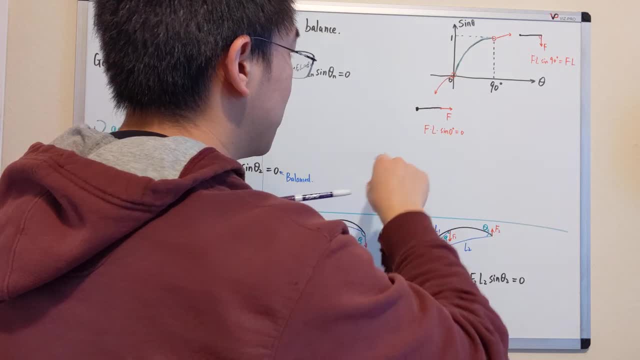 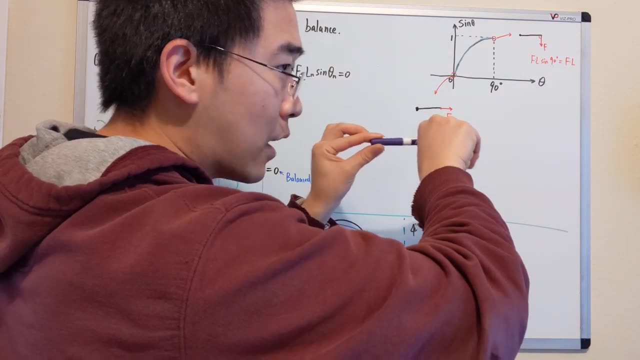 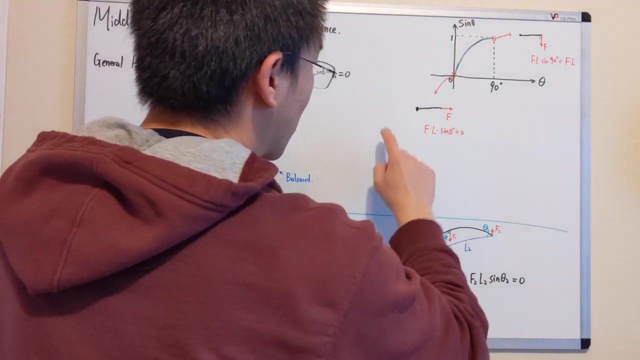 and we give it theta equal to zero, which means the line is parallel to the force. So we basically give like this: As you imagine, it doesn't give the lever any tendency to rotate, so there's no torque. And on another extreme spectrum, 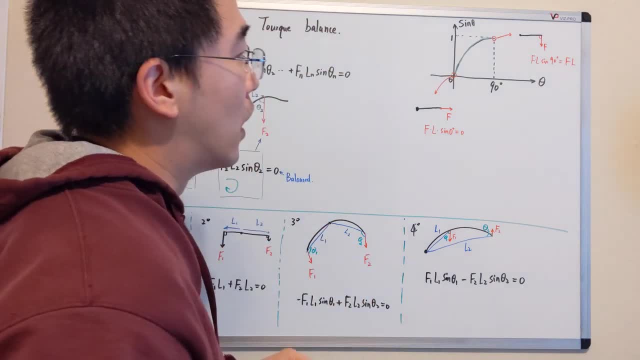 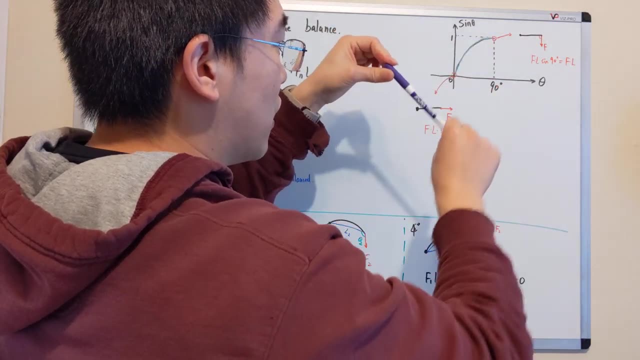 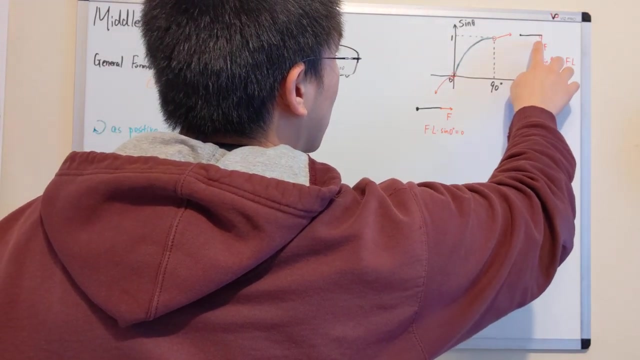 we have a sine Theta equals 90 degree, which is the lever perpendicular to the force, Then you can imagine, if we put any force down, then this will rotate clockwise. Then all of those torque being used, there's no waste. So since the sine theta, sine 90 degree, is one, 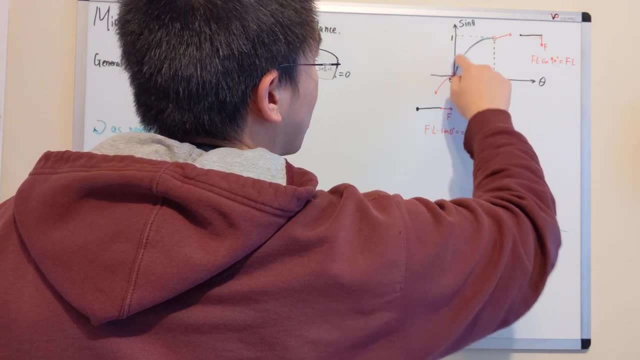 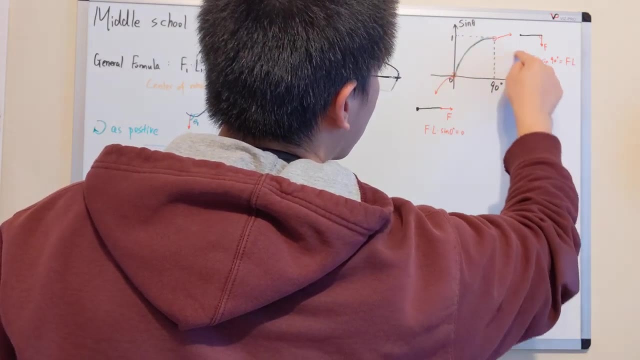 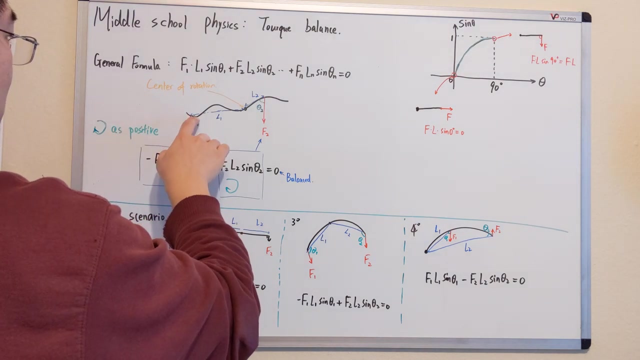 So, as you can imagine, as you remember, our sine theta is a symmetric from zero to 90, then it's from 90 to 180 is the same, but just like a mirror on this way, which means, if you take the angle like this, theta 1,. 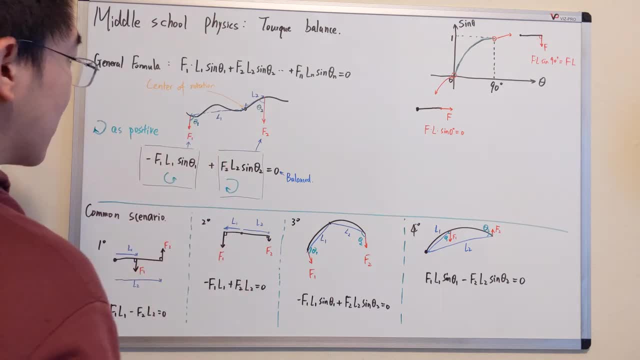 or take the angle of 180 degree minus theta 1, it's the same. It's the same number, like this. So most commonly we have four different scenarios. Technically we only have two scenarios, But let me just start with the easiest to the little bit harder ones. 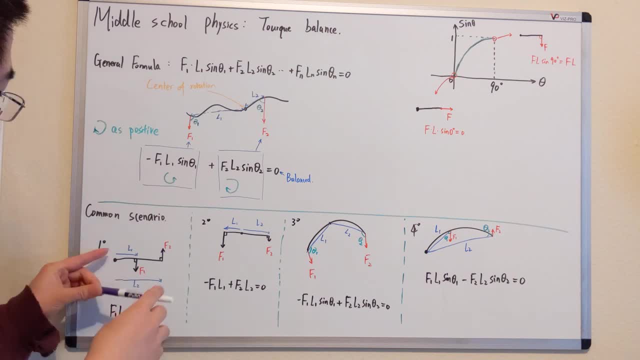 So the first scenario: we have a lever, The center of rotation is on one end, The force is going down, F1 is pushing it down, The F2 pulling it up. So, as you can see, as we do the same thing, 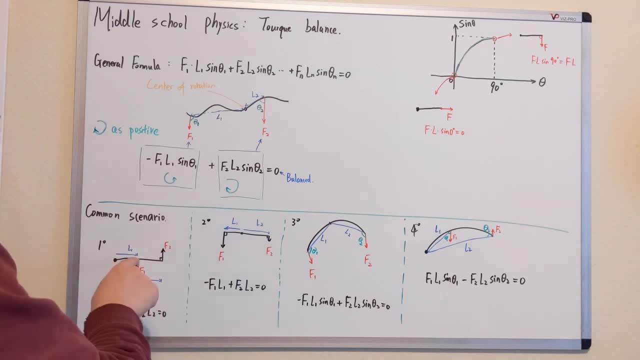 the center of rotation, the point of force is acted. The line is L1, same to the F2.. The line length is L2.. And as you can imagine, as you can see that the L1 and F1 is perpendicular. 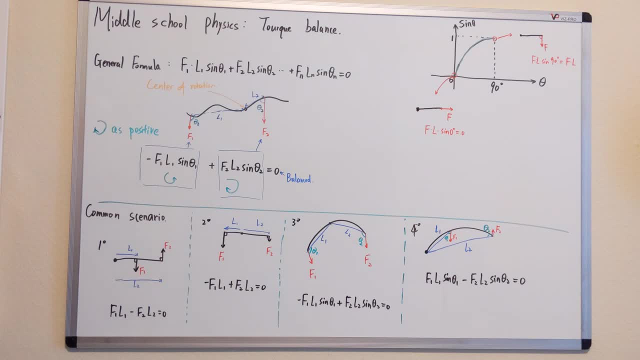 And sine 90 degree is one, So we just spare ourselves with calculating the sine theta. Okay, So now we need to determine the sign of each term So we can imagine the force going down. This pen will go clockwise. That means, as we define the positive, clockwise. 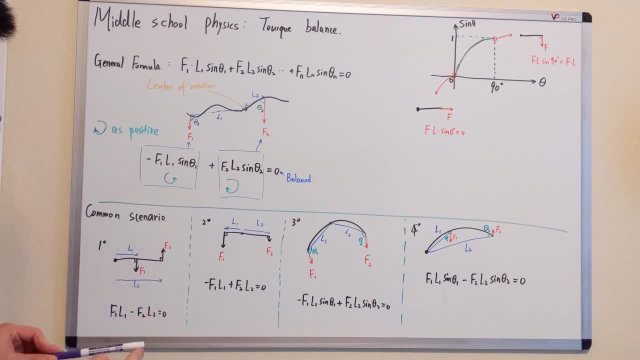 this term is positive. On the other hand, if you're pulling it up here, the pen will go counterclockwise. Then this term will be negative. So we end up having F1 L1 minus F2- L2 equals zero. 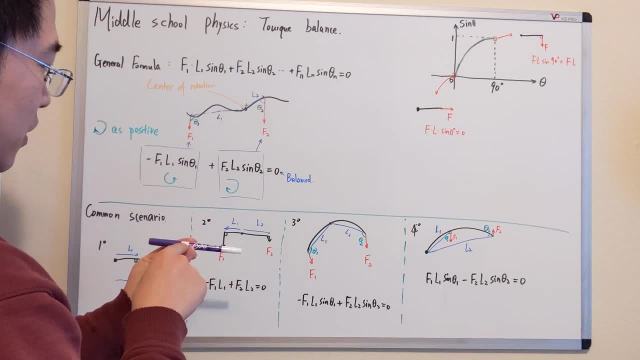 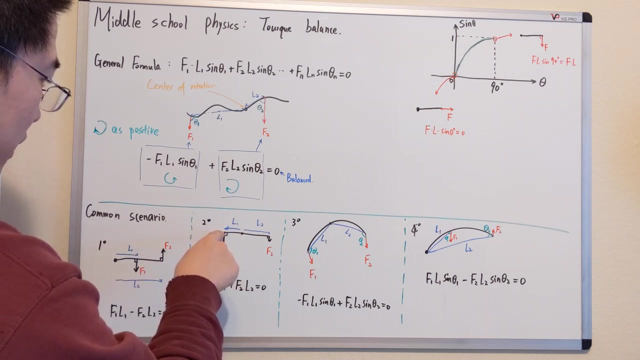 And in scenario two, we have center of rotation in the middle And we push it down on one side and push it down on the other side. Same deal. We have center of rotation where the point of force is acted here and here. So the length is L1 and L2.. 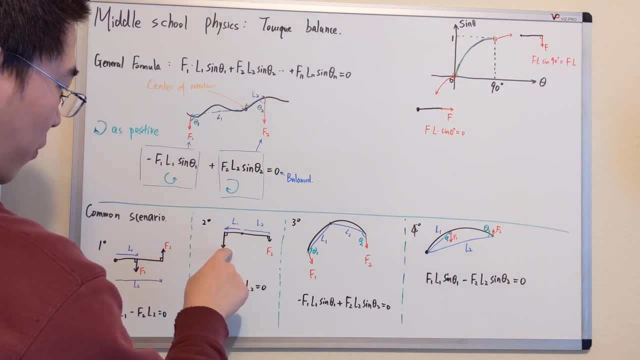 So again in this scenario we have: L1 and F1 are perpendicular to each other, L2 and F2 is perpendicular to each other, So we don't need to worry about sine, Sorry, the sine theta, Since sine theta is one. 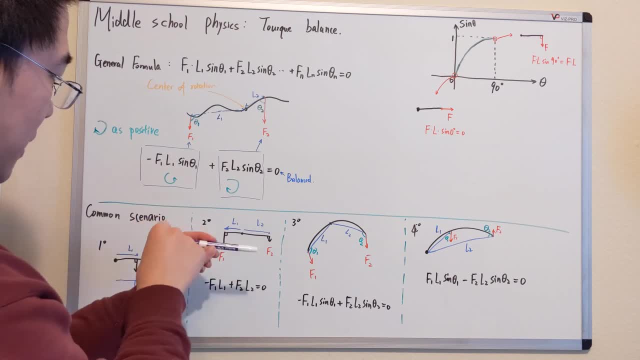 And if you imagine, if you push it down on the left-hand side, the pen will tend to rotate this way, which is counterclockwise. So it should be negative. So negative: F1- L1.. And this will be positive: F2- L2.. 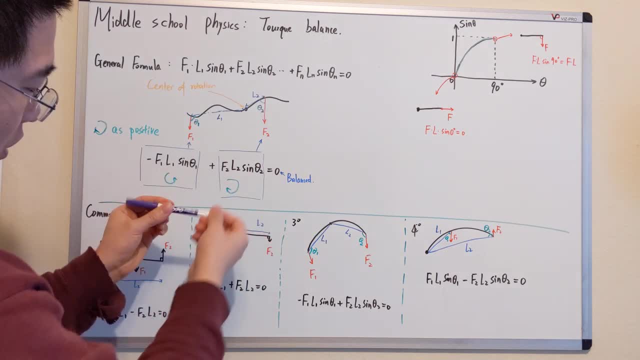 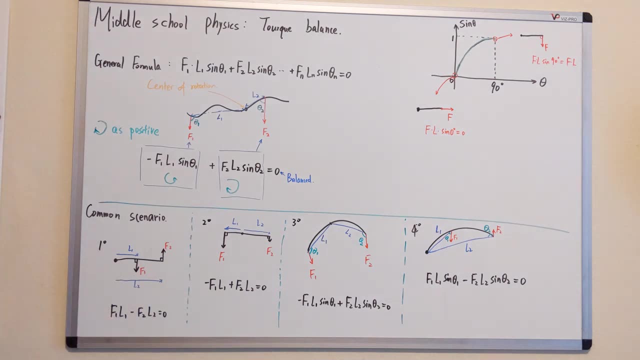 So, since you can see this, it will go clockwise this way: Then it will be minus F1 L1, plus F2 L2.. So this and this is a similar scenario, but with angle and the not straight lever which is added to the complexity. 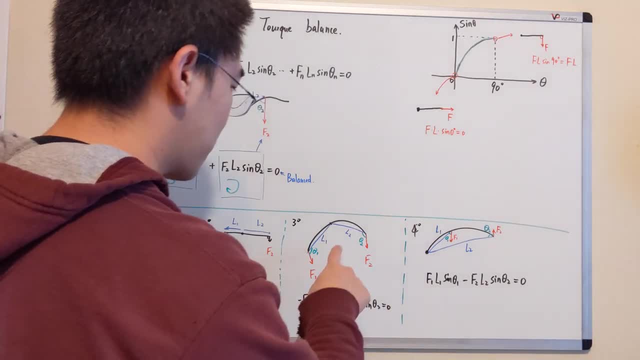 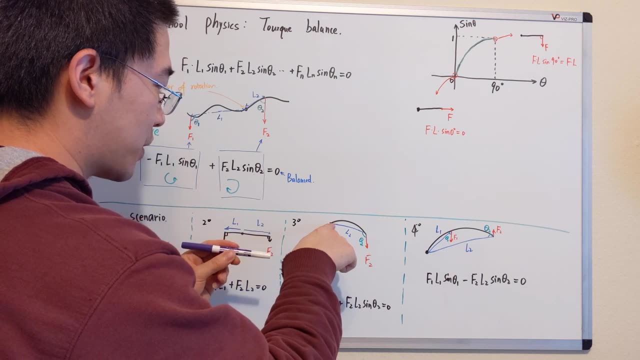 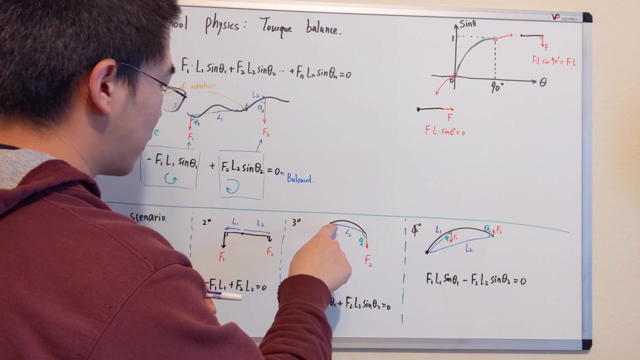 And those two are pretty similar. So let's look back, Look to this. So we have a lever that is banded a little bit And we have a center of rotation here And force F1, force F2. And we connect the dot of the center of rotation. 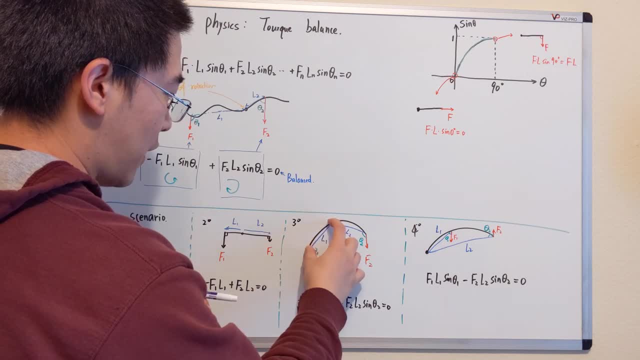 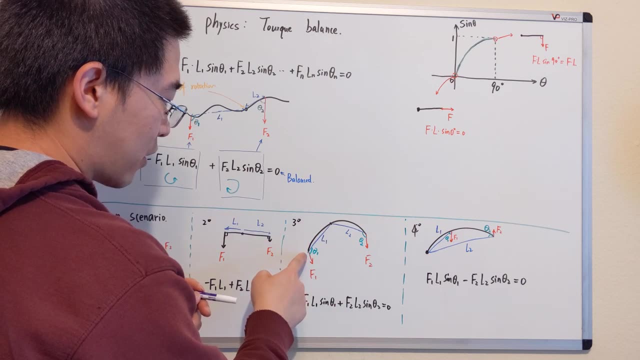 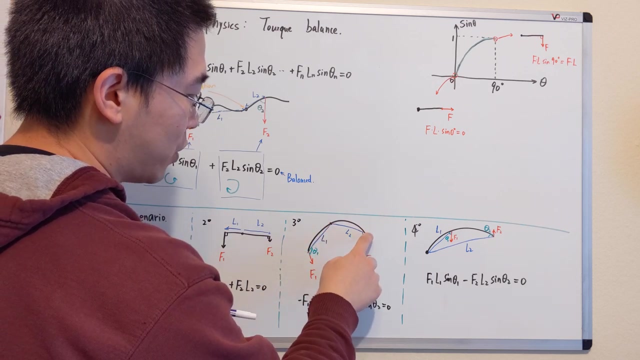 and where the point, the force is acted. This length, this straight line length is L1.. And the L1,, the line, has an angle with F1. That angle is theta 1.. Similar here: Center of rotation F2,. 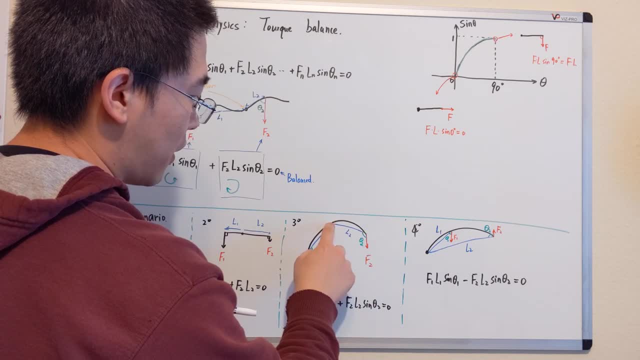 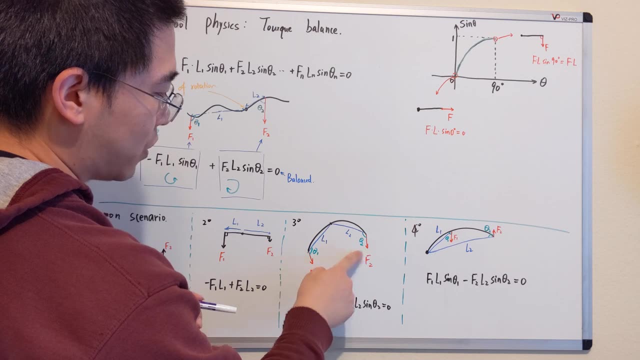 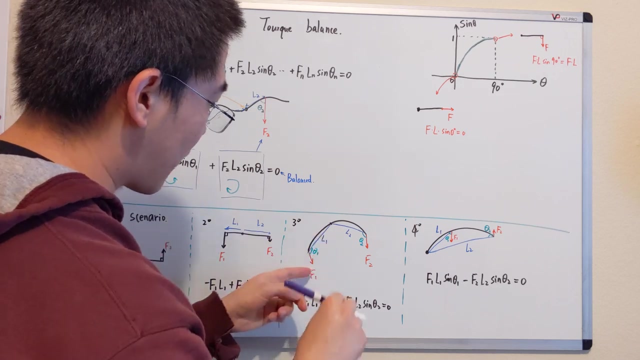 the point where the force is acted, F2.. The length will be L2.. The L2 have angle with F2. It's theta 2.. So now we need to determine the sign of each torque. So this, if you can imagine: 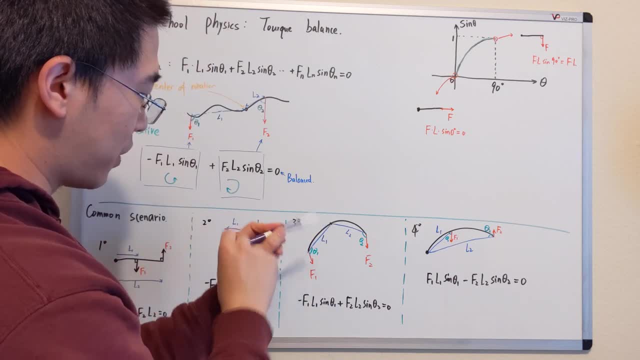 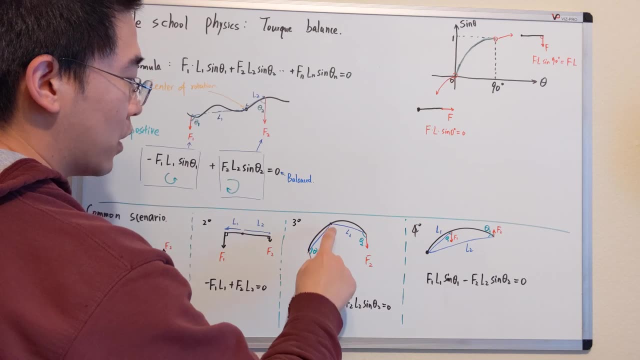 it's going. if you apply F1 here, it will rotate counterclockwise. So it should be negative. So it would be negative. F1 L1.. Sine, theta 1.. And this will go clockwise if you apply force down on the right hand side. 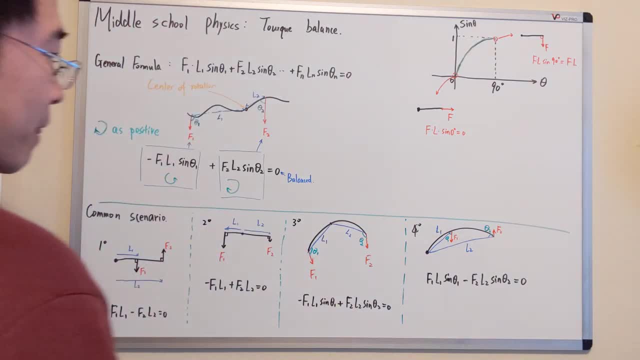 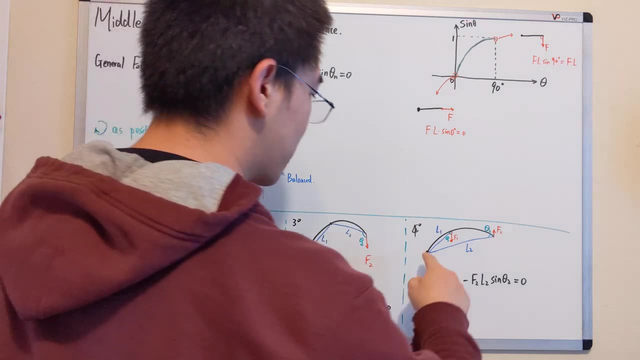 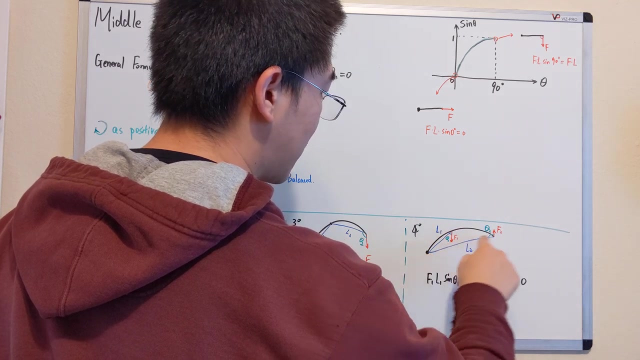 That will be plus F2, L2, sine theta 2.. So the last one, we do the same thing. I believe now you already know the drill: Connect the center of center of rotation where the point of force is acted. Center of rotation, force is acted.